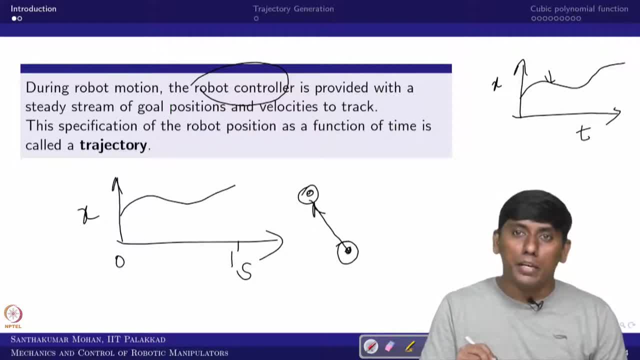 you need to actually, like, identify some kind of predefined path, or you call trajectory. So why this is required? because sometimes there would be obstacles, So it need to go. or probably in order to make the energy optimal or time optimal, So you need to have some. 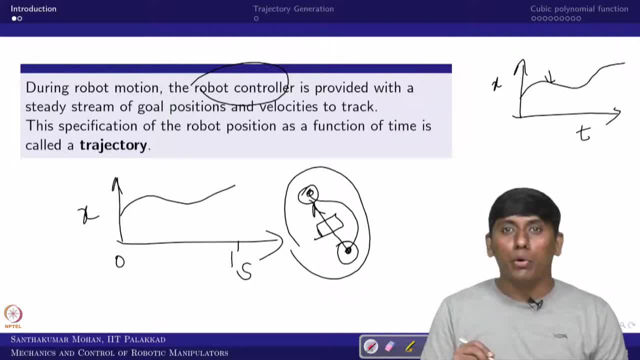 predefined manner of you can say, following one point: So this is what the prerequisite. and when you talk about controller, So you have all the time actually like some desired and you have actual, So you are actually trying to compare and trying to maintain the Q actual become Q decide. So this can be actually 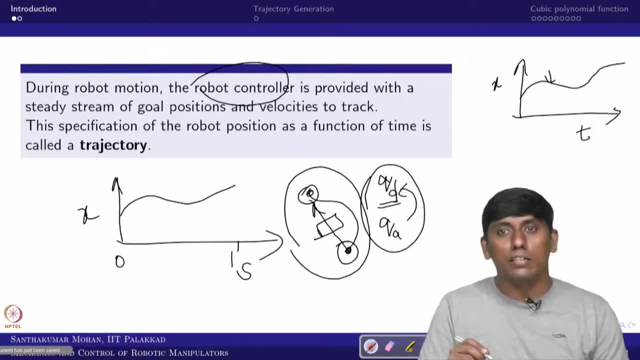 like just a constant. For example, you take a air conditioner, you keep 20,, 22,, 24 or 16.. So these are actual like set right. So then the air conditioner supposed to follow this in a, you can say, piecewise manner, whereas you assume that you are actually taking a. 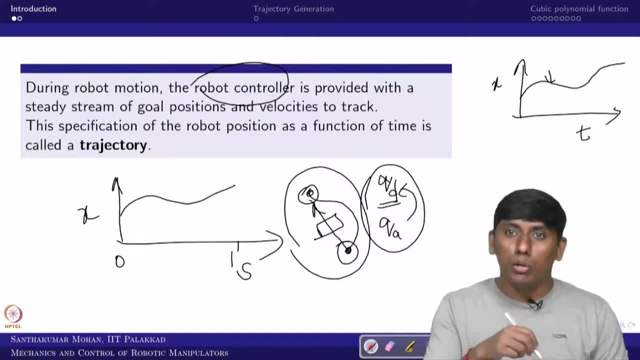 probably a milling machine or you actually like trying to draw a diagram, So then you actually follow certain manner, right? So then this is actually like each and every time, would be actually like define So these all we are trying to see. that is point. 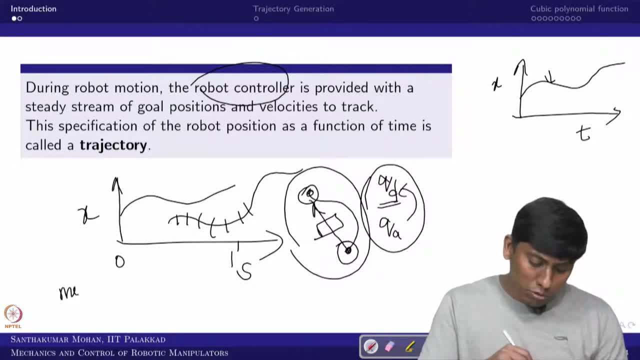 we are actually bringing it here. So now we are talking about the motion, Tips 2. Motio, So the motion is actually like what we define Mai Maude 最近 We bother about, actually like the position and its derivative, which is actually like 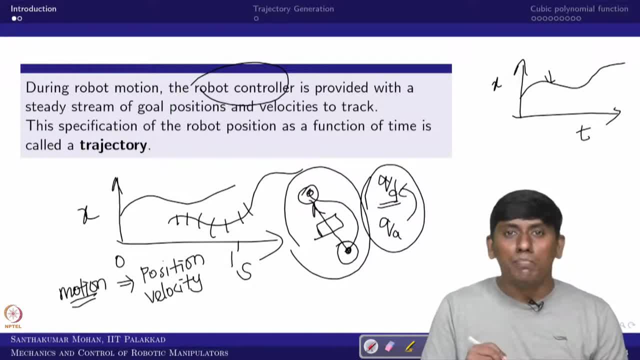 velocity. So these two things are very important, even if you are going for a dynamic level. even the desired acceleration also important. So then you can see like: so acceleration is the third part which we are bringing it. So in the sense, we are actually like trying to see these all. 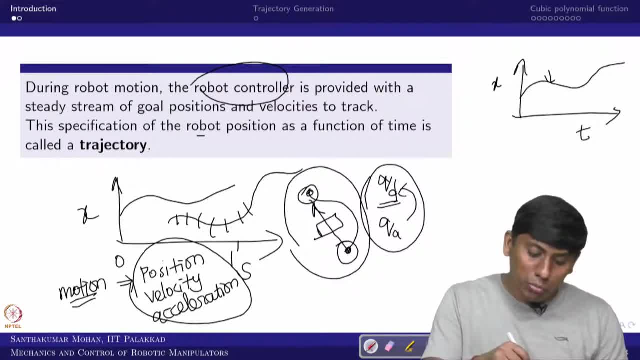 So for that, we are actually like going to specify the robot position as a function of time. that is what we are going to call as a trajectory. ok, So now you can actually like understand. the trajectory can be given one way of definition. it is nothing but specification of a robot position as a function of time. that is what. 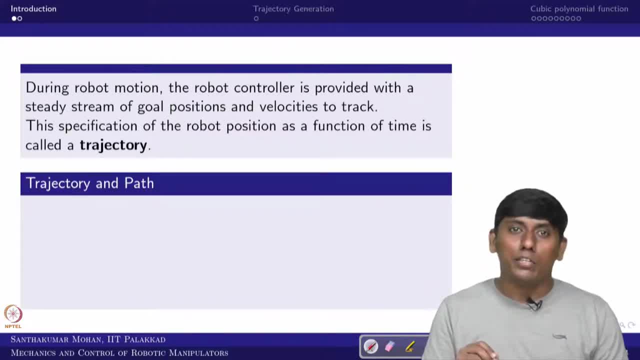 we are calling trajectory. So then we need to actually like differentiate what is path and trajectory. So for that we are actually like taking the trajectory means, so we take q is the you call the position. So the q of t is actually like given where it is starting from. 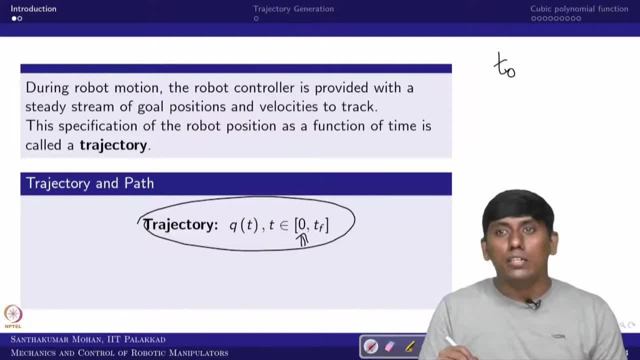 It need not to be 0 all the time. so I said that starting point is t0 and it is actually like ending as tf. So where I define this q as actually like t, so the t vary from t0 to tf. So this is what we call trajectory. so in the sense is it time dependent? in the sense? 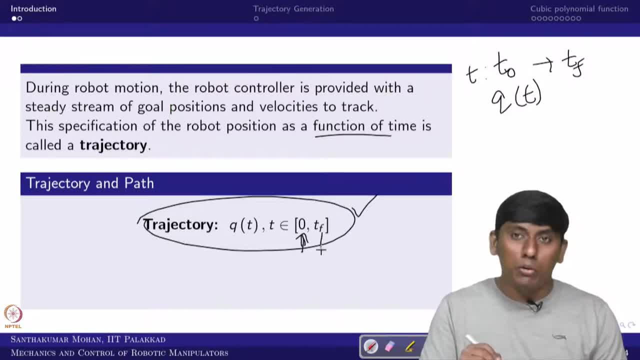 you can see it is a function of time. Now this tf and t0 I actually like converted into 0 and 1 and this I actually like call q of s. So where there is only you call subset of s. that s actually like vary. you can say 0. 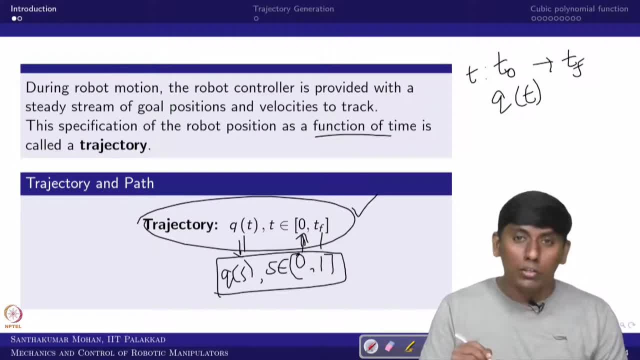 to 1.. So if I make this, you see there are time dependency is gone and you no need to actually like bother. even it can be easily scaled up to any given time range. So this is what we call actually like path. it is need not to be function of time. 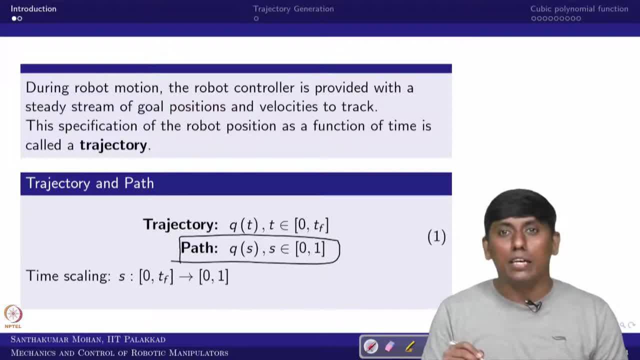 So that is what we are calling like path. we can actually like rewritten as another set of function, So q of s, where s actually like belongs to. or you can say s is vary 0 to 1.. So how we convert the t0: we equal to 0 and the tf, or you can say tf minus t0, so that 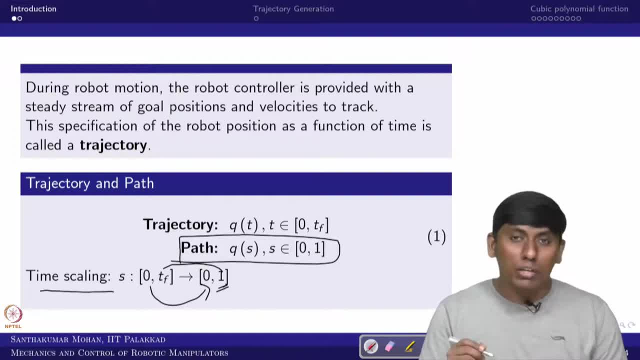 we are actually like equating to 1.. So now this is what we call time scaling. So most of the cases we do the time scaling. so because the path, easily we can generate with respect to 0,, 1 or the s is varying 0 to 1, that way we can generate and we can actually. 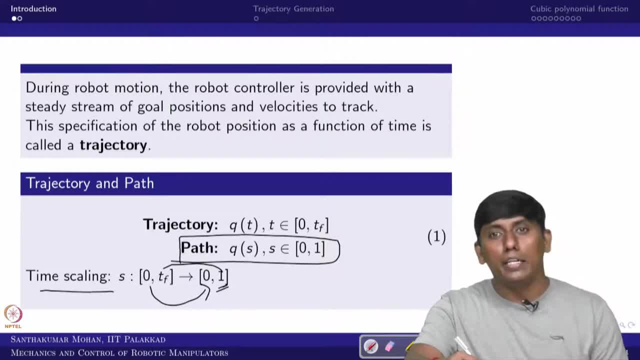 like scaled up whatever way you want. For example, now my end effector supposed to move in 10 degrees per second as the you can say speed. So then I can see what would be the time required. I want to actually like increase the speed of that system. then I can actually like change the time step, like that I can. 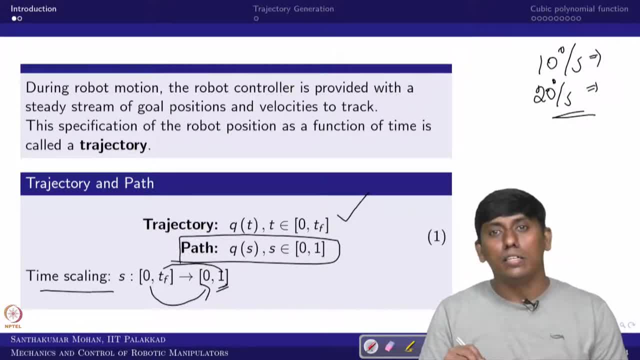 make it. So that is what the whole idea here we are insisting, the- you can say- robot position as a function of time. that is what we are focusing as a trajectory here. Ok, In that sense. so either you call Q of t or Q of s. that should be at least twice differentiable. 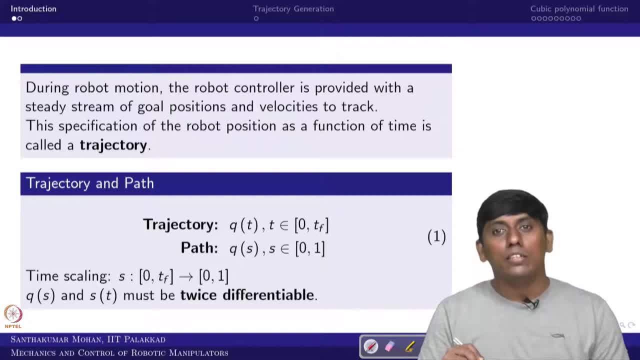 in the sense. the acceleration is definite in the sense. So acceleration is actually like what you call finite value, or it is function of time. it would be there. So in that sense, your actuator will start in a proper way. So that is what we are actually like putting it. 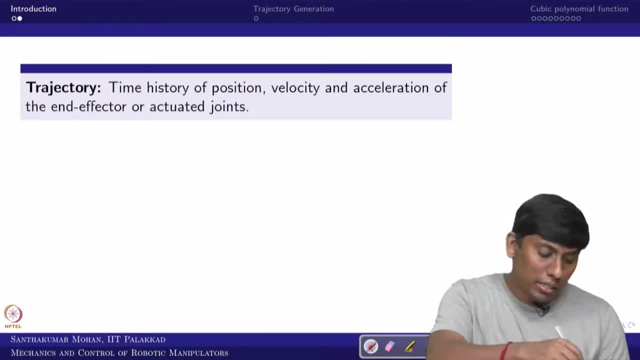 So in that sense we are actually trying to see little more in detail So what that means. So we are again bringing back the different definition. So you should actually like, should be familiar. So the trajectory is nothing but time, history of position, velocity and acceleration of. 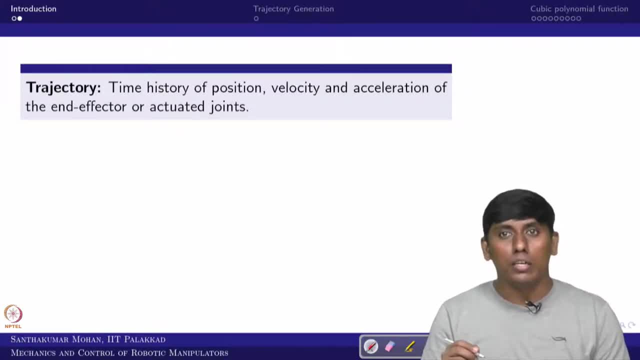 the end effector or sometime it would be actuated joint. It depends on what space you are actually like working on. So for example, you are working on a configuration space, then the you can say time history of you can say actuated joints in the sense joint position, joint velocity and joint acceleration. 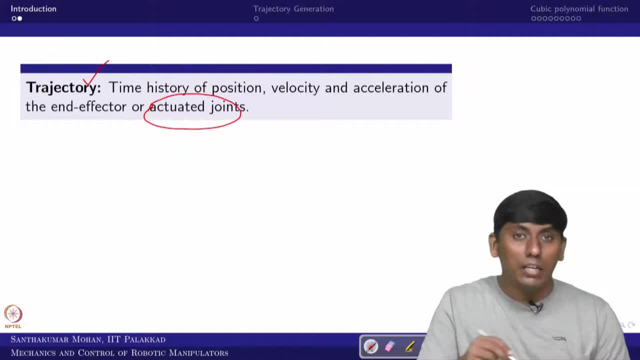 we write in time, Time history. that is what you call trajectory. or you are actually like bothering about the operational space where the end effector point, you can say the position, velocity and acceleration need to be generated. then that is actually like end effector trajectory. 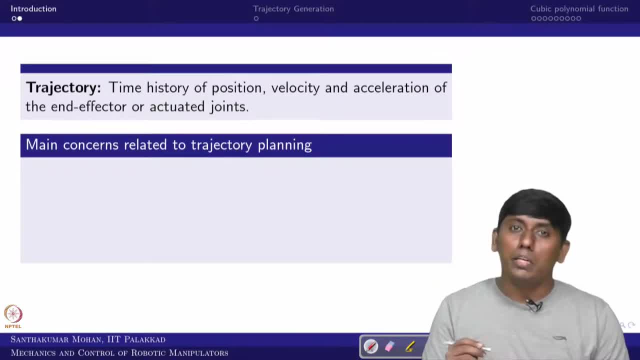 So that is what we are seeing it. So in that sense, what would be the main concern? So already I said it is supposed to be twice differentiable. But what if you are thinking about in terms of real time implementation? So one is ease. 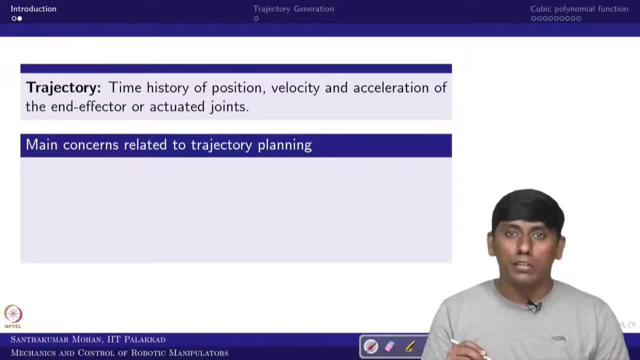 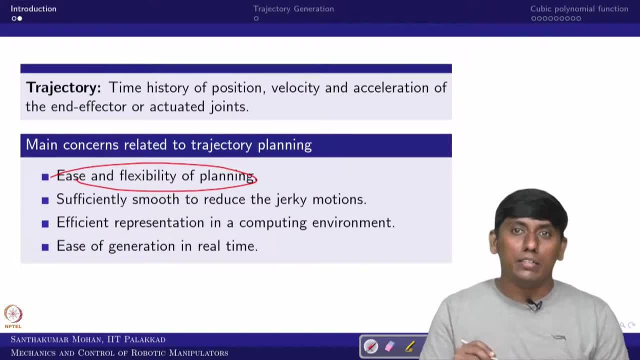 So it is supposed to be ease of generating and it should have a flexibility. So that is one important point we need to think about further. So when you generate any trajectory, the trajectory should be very smooth, So in such a way that the robot manipulator or even robotic system that should actually 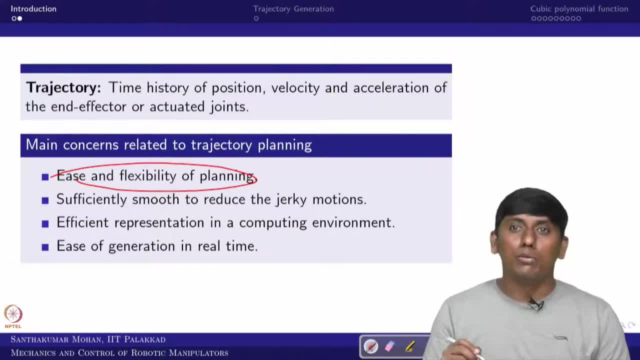 like take away from the jerk. So, for example, now you take a car and you start and you actually like release the clutch arbitrarily, So what happen? there would be a small jerk, right. So how about you? However, if the experienced driver, you can see that there would not be any, you call jerk. 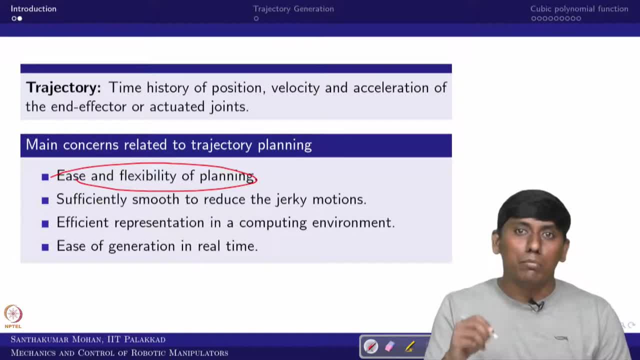 you can experience when the car is starting right, when start moving. So that is what you call the smooth trajectory. So in the sense, your trajectory should be smooth so that you can avoid the jerky motion in invariantly. it will actually like reduce the cost of, you can say, overall system and 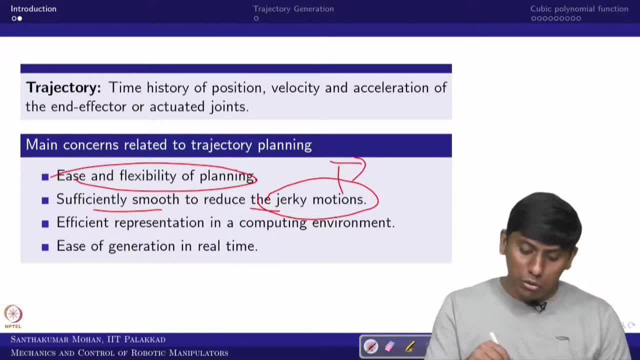 long life of the actuator will come. So that is what the whole idea. So further in terms of attraction, So in terms of actually like real time, you can say- computational point of view, So it should be efficient. So the representation of the algorithm or the trajectory planner should be efficient. 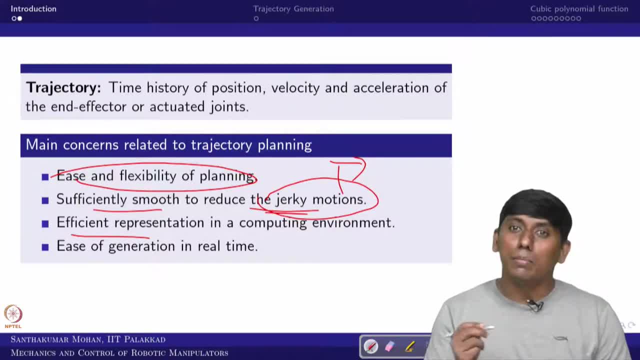 and as well as it should be actually like fast enough, in the sense, the processing time for computing should be actually like good. So that is what we said: ease of generation in real time, So that you can easily implement it any point of time. that is what the whole idea. 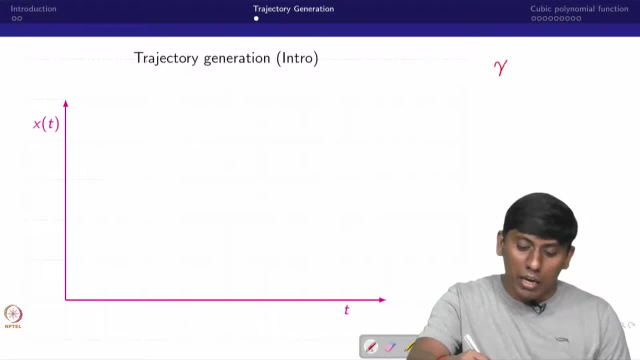 So just to take that. So what would be the easiest to understand? So I have x of t, so that is actually like varying x0 to xf. I am just saying. So this is corresponding to t0 and this is corresponding to tf. So what would be the easiest to one? 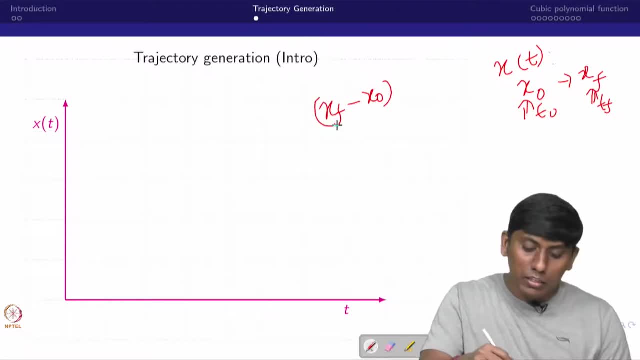 So we will say that what is xf minus x0? okay, So this is actually like tf minus t0.. So this I call as a slope, in the sense, linear interpolation. So then I will actually like take it as a function of time. So this would be x0 plus this. 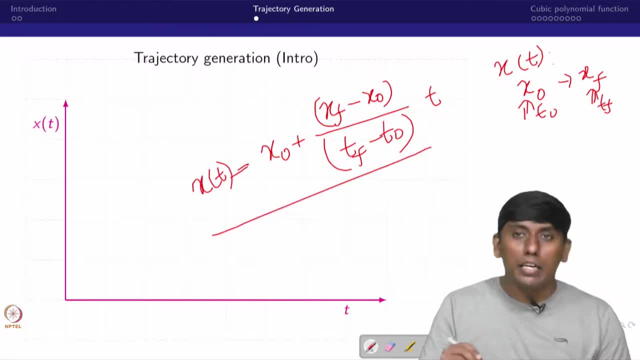 This is y, This is what x of t. So now, in that case, what it is giving? it is giving a linear interpolation, But this linear interpolation is giving what? So it is actually like giving a constant velocity generation. If you think about constant velocity, what would be the acceleration? 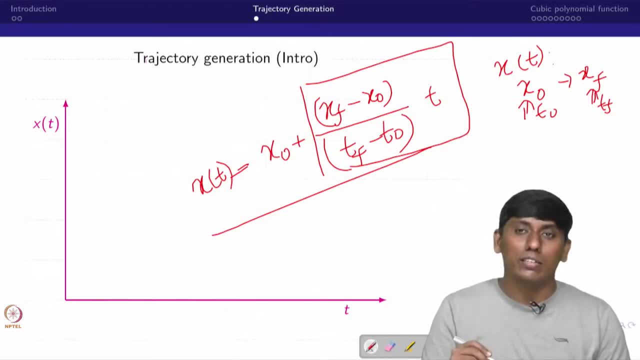 So it would be infinite in both acceleration and deceleration at initial and at the end. also infinite deceleration and acceleration, right in the sense. So your acceleration at initial and the end point should be infinite, Which is not possible. you do not have a smooth curve. 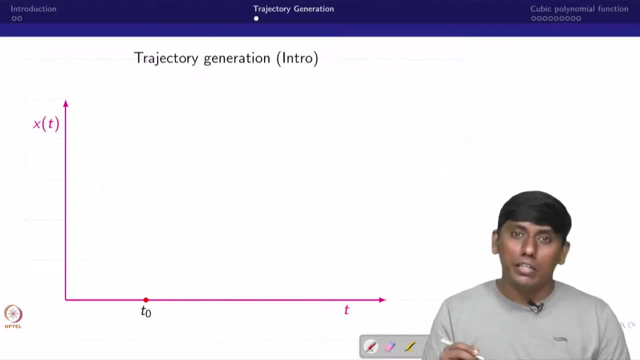 So for that only, we are actually trying to see. So whatever I have written in actually like analytically, So that we can see in symbolic or you can say, graphical manner. So this is what I said, the initial point and this is the final point of x, of t. 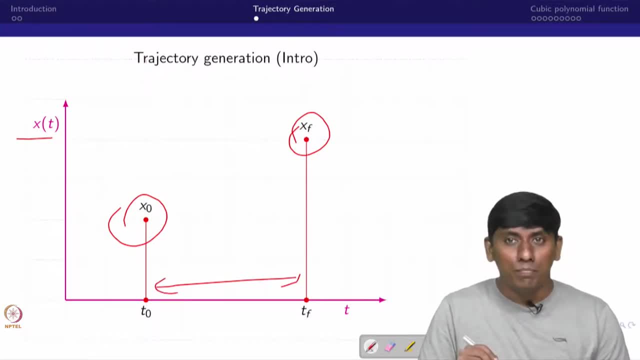 And this is their duration which I want to actually like see. So what is the one of the easiest one? I connect as a straight line, Which is actually like really a better one, But what happen? the velocity would be a constant. When I actually like draw time versus, I start t0 to tf. 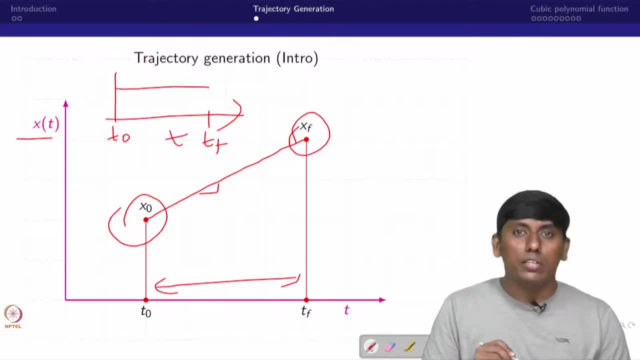 So the velocity would be constant, right. So if the velocity is constant, what would be the acceleration? So the acceleration would be so infinite acceleration and deceleration. So similarly here it would be. So that is actually like little constant for us, ok. 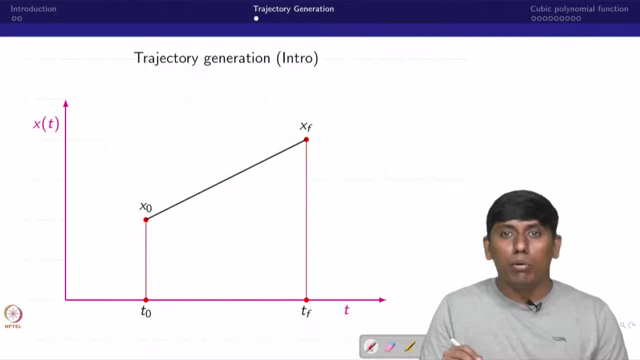 So this is actually like velocity and acceleration. So in order to avoid that People are actually like thinking about this is what the linear interpolation, So in order to actually like get this, So the t0, we always assume 0. So what, if it is t0, is there? then you have to actually like substitute that. 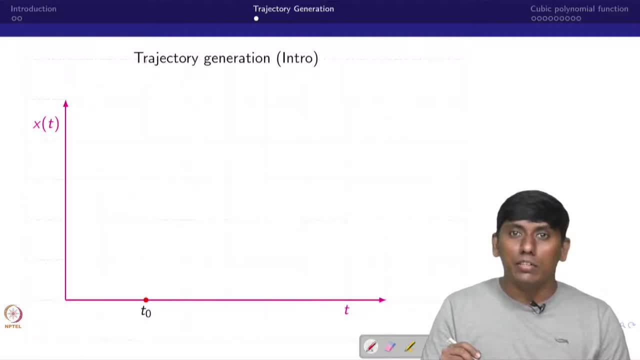 So not simple t. So I will just rewrite this equation: So this is actually like minus t0, ok, So that you can actually like get it clear. So now, in that case, So what we are actually like writing this is linear interpolation. 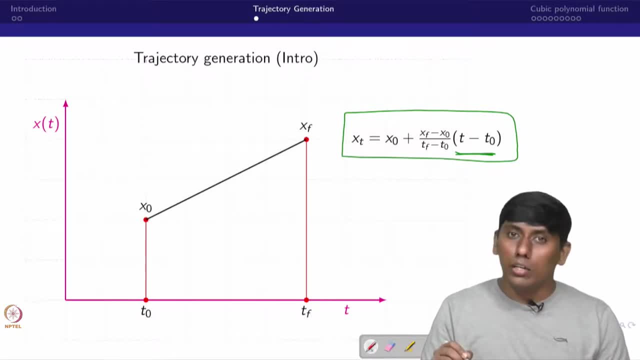 This is not smooth, It is actually like a jerky motion. So, in order to avoid what one can see, So there are actually like several possible. You can see, these two points can be connected like this. ok, So like this, and there are several possibility to reach from this. 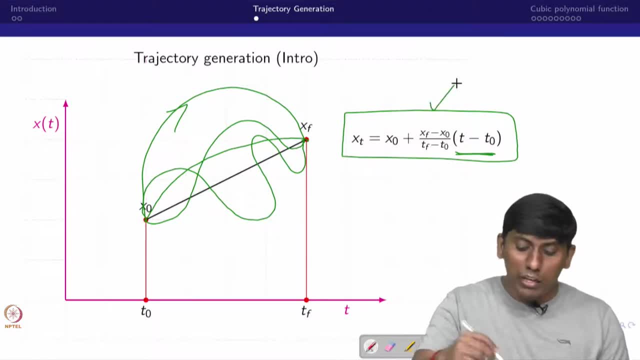 So we are trying to see what would be the efficient. So this is actually like first order. The second order is possible, which is what you call the quadratic equation. but quadratic equation So we are having, so the number of you can see equation and number of unknowns are actually 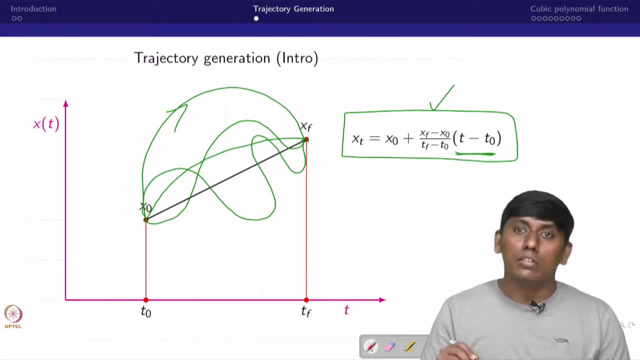 like not properly matching. So we will go with. you can say cubic polynomial. where the cubic polynomial, the equation. I can write: So: a0 plus a1 t plus a2 t, squared plus a3 t, cube, where t0 I assume as 0.. 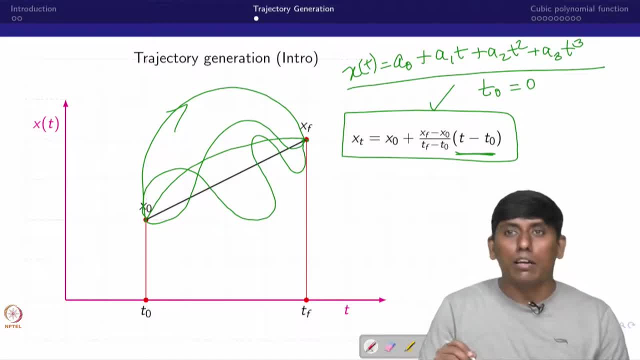 So which is I called this? So, in the sense, what you can see, there are 4 unknowns. So this 4 unknowns, 2, x of 0, x dot of 0, I can equate, and similarly x, you can say x dot of t f and x of t f I. 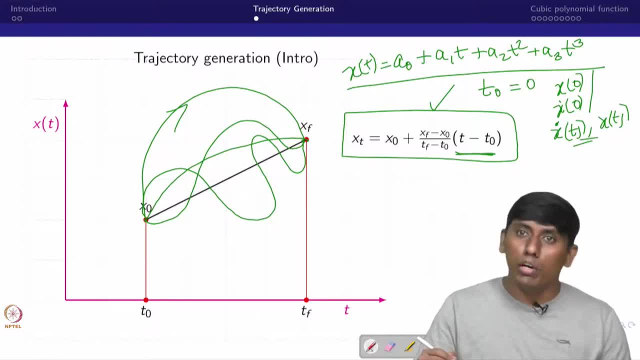 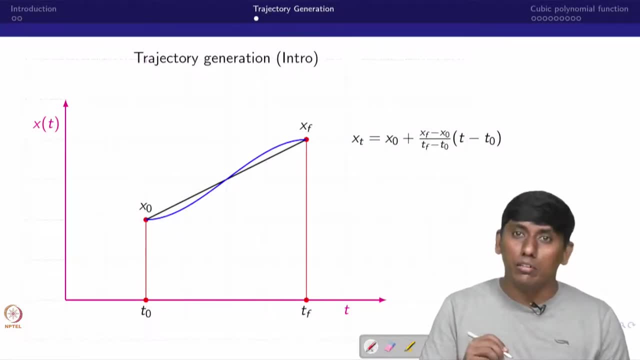 can actually like substitute, you can see. So 4 boundary condition and 4 unknowns. I can get it. So that is what we are trying to see. So, in that sense, the cubic polynomial which I have shown, it is very smooth, So which is actually like very close to what? 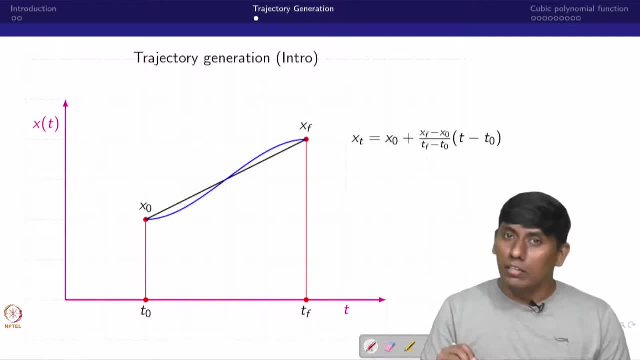 you call the straight line, but it is actually like very smooth, It is actually like going to give at least twice differentiable. in the sense the acceleration would be finite. So that is what we are trying to see here, So in the sense, what one can see, this is what 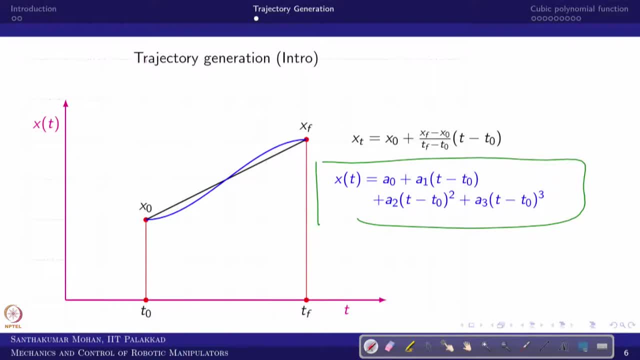 the equation which we generated. So in that sense you can actually like see. So these 4 unknowns we can actually like calculate by bringing the, you can say 4 conditions. So I call: this is x naught and this is x naught. 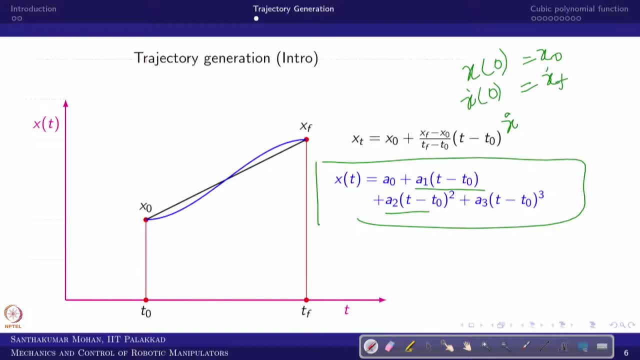 So this is x f and the x- sorry, this is x dot of naught and this is t f. So then x t f is called x f. So in the sense of 4 unknowns and we can actually like get, you can say 4. 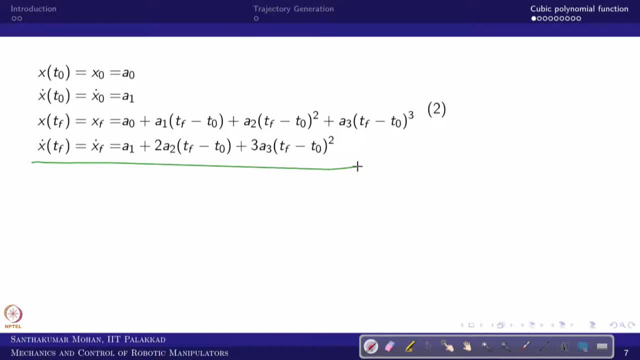 equation and then we can solve. So that is what we are trying to write it here. You can see: further you differentiate. So what will come So further if you differentiate? So it would be actually like: further if you differentiate. So the equation x of t is actually like: 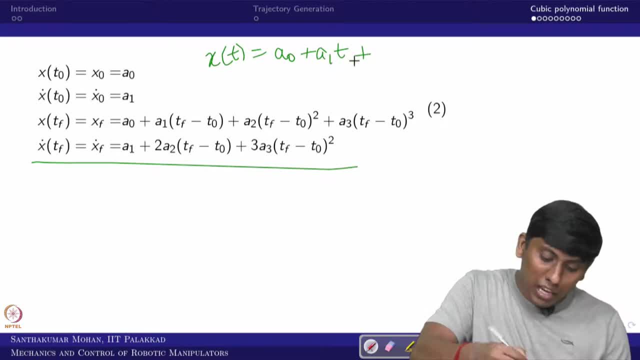 So a naught plus a 1 t plus. I am just assuming that t naught is 0. This is explicit assumption here. Otherwise I have to write t minus of t naught. So in order to avoid that, I am writing: So what would be x dot of t? that would be. 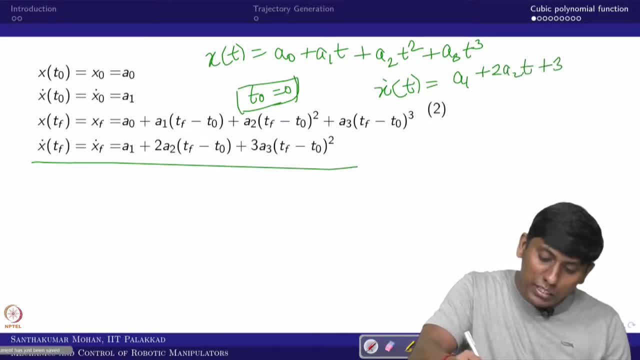 a 1 plus a 1 t. So what would be x dot of t? So what would be x dot of t? that would be 2 a 2 t plus 3 a 3 t square. What is the x double dot? So that would be So 2 a 2. 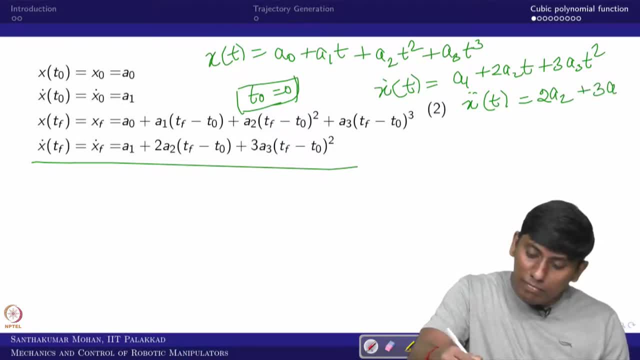 plus, you can say 3 a, 3 t, right? So this will be sorry, this is 6.. So this will be coming, but you need actually like only 4 equation. So we will actually like take this and this and we can actually like substitute and you can do it. 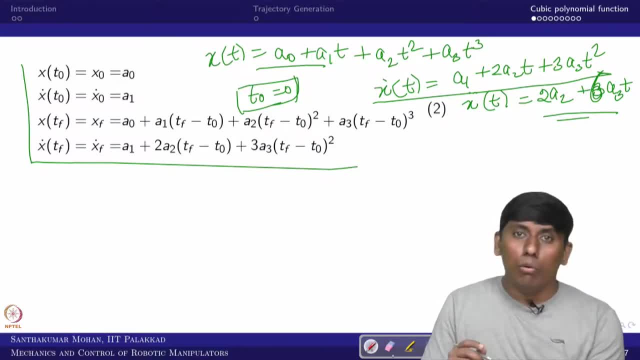 So now for solving this. there are several way. So one of the easiest way, what we can do it: we can rewrite this in a state space form. So what we can do, So we can write the unknown, So so a 1, a naught, a 1, a 2, a 3, or I can write it to one side and the other. 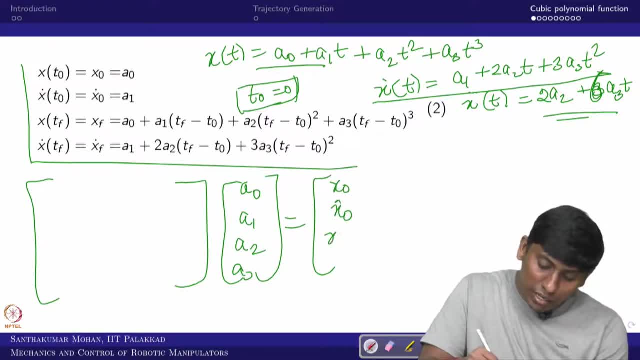 side, actually like x naught, x dot of naught and xf, xf dot. I can write, And you can see the first equation: it is 1 0 0, 0.. The second equation is there, So I can write it as a. 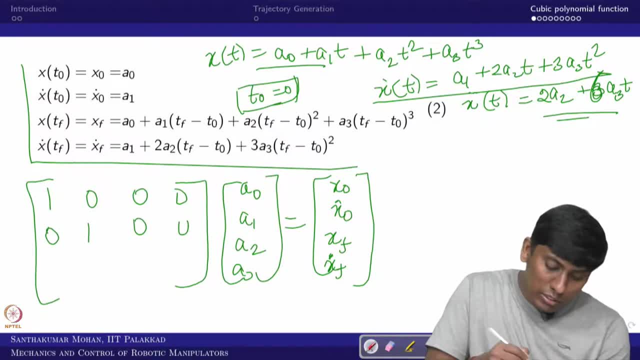 1 0 0 0 0.. The second equation is like this, So I can write them as a 1 0 0 0 0.. I can second equation 0 1 0 0 and the third equation 1. then you can see tf minus t0 and tf minus. 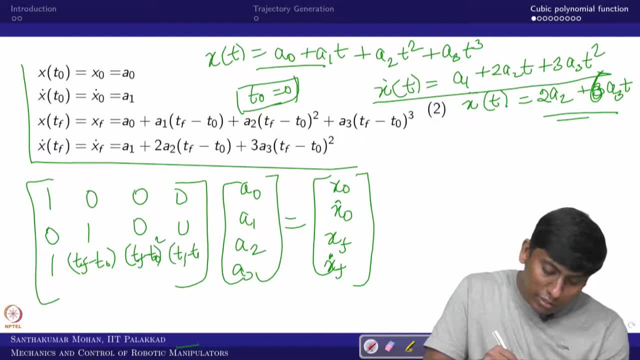 t0 squared, and the third one is tf minus t0- cube, and the third one 0, 1 and 2, so tf minus t0 and this is 3 tf minus t0, square right. So now this is actually like linearly independent. you call rows containing 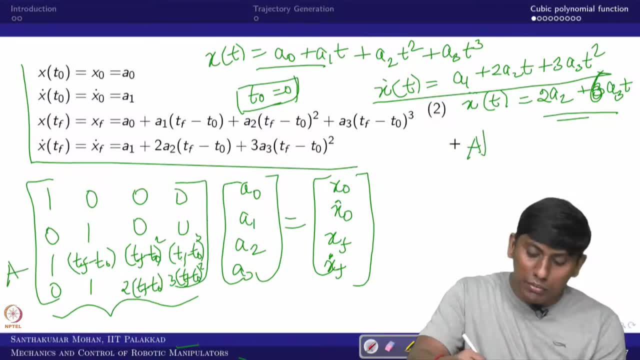 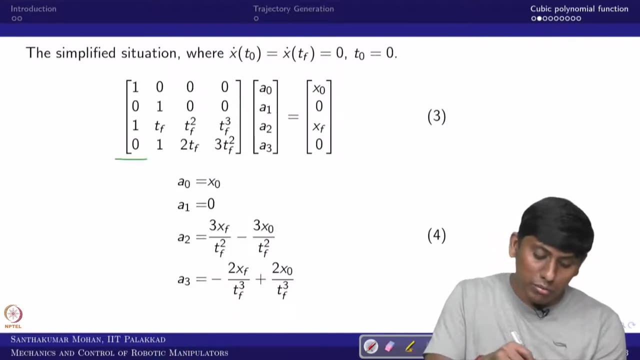 So in the sense, this I call a, so the determinant of a is actually like non-zero, okay, So in that sense, what one can see? so if I take inverse of this and multiply with this, so that will give a0, a1, a2, a3. so that is what we are actually like doing it. 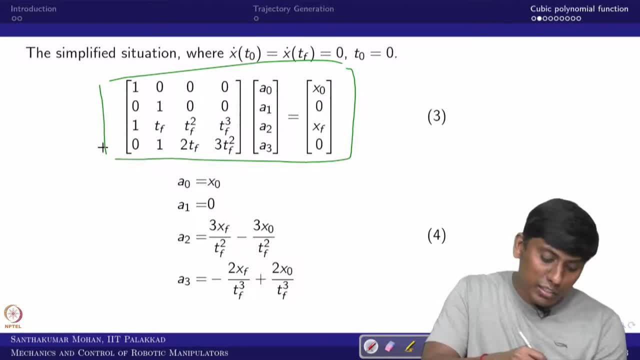 So you can see, I take this, I take this a inverse, So this a inverse, I multiply with this and I can do for making a simplification. I assume t0 is 0 and initial velocity and final velocity are 0.. So in that sense, what happened? x dot of 0 and x dot of f, both are 0. 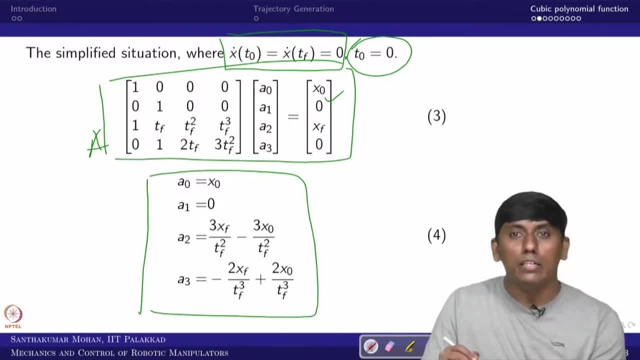 So which gives the a0, a1, a2, a3 in a simplified manner. okay, So the same way, you can actually like, even you put it non-zero value, but t0, we can make it always 0. Because we can actually like bring it t0 at the end wherever it is required. 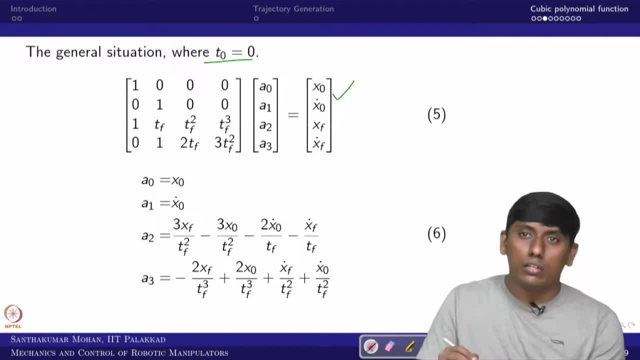 So in that sense you can actually like assume x dot of 0 and x dot of f are exist, So then the a0, a1, a2, a3 are obtainable in this way. So now you know all the coefficients. once you know the boundary condition, then what? 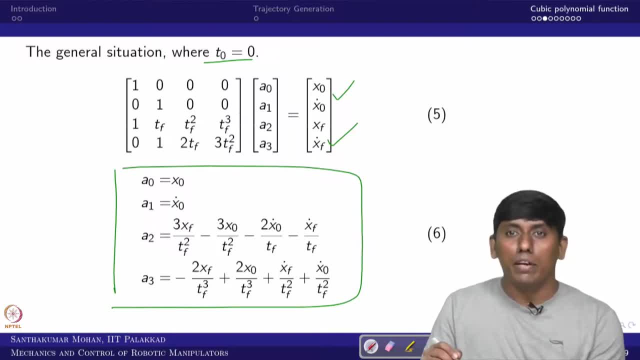 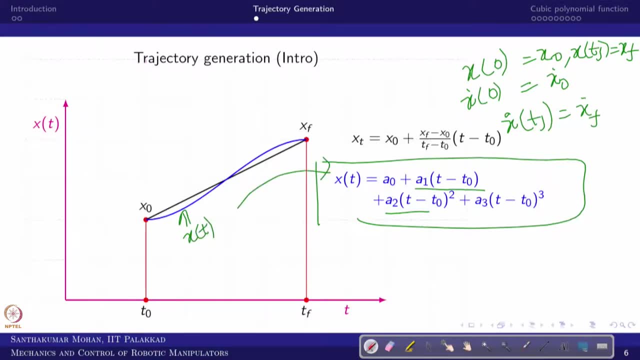 you can do, you can actually like generate the trajectory. So that is what we have done in the here. So this is what you call x of t, Okay, Cubic polynomial. So now this equation actually like arrive. So now we will actually like go back. individual component. 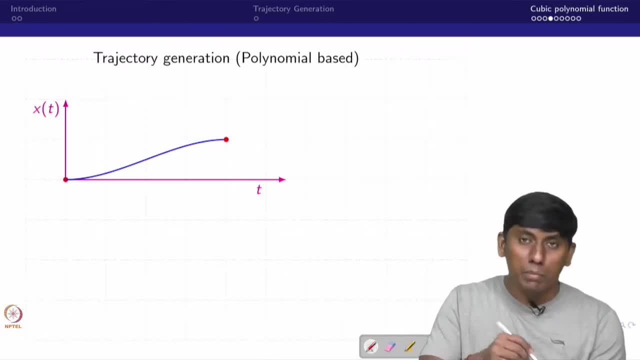 So in the sense how the velocity, how the acceleration will come, because the position profile we have seen. So now I assume that it is scaled down to 1.. Okay, So in that sense, t0, I assume 0 and tf. So this is the duration and the s displacement, or you can say x of t as the, you can say displacement. 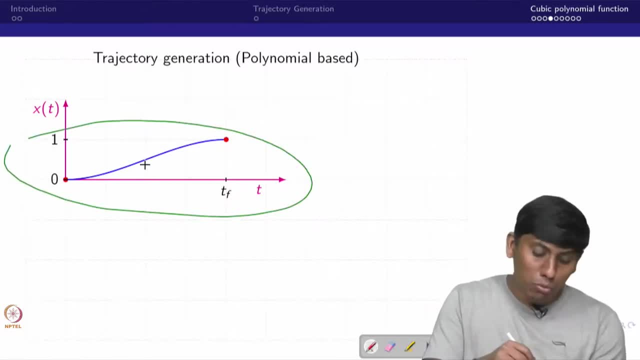 as 1.. So then you can see the profile. it is smooth, smooth. So now if you rewrite this into a velocity form, you differentiate, you can see the velocity would be maximum at the middle of the duration, So that the value would be equivalent to 3 into 2 tf. and even you bring the non-zero initial condition, all those things, 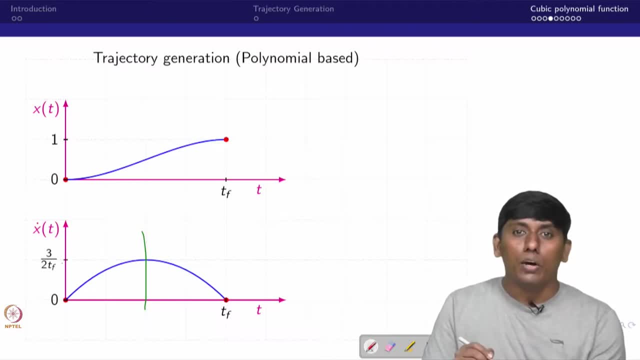 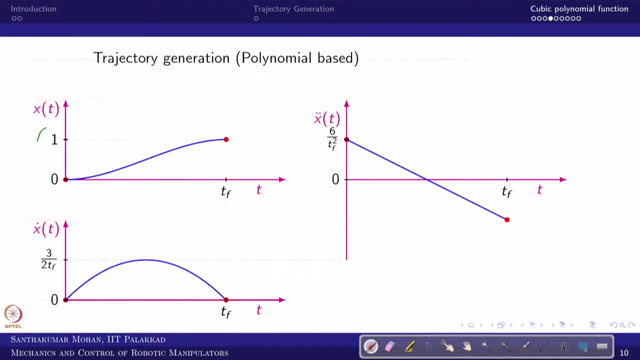 will come. theta f minus theta 0 would be added okay. So now, the same way you go to acceleration, you will feel a little strange because the acceleration will start from non-zero value, okay, and similarly end with non-zero value. So now we assume that this is actually like 1, so based on that, you can actually like see. 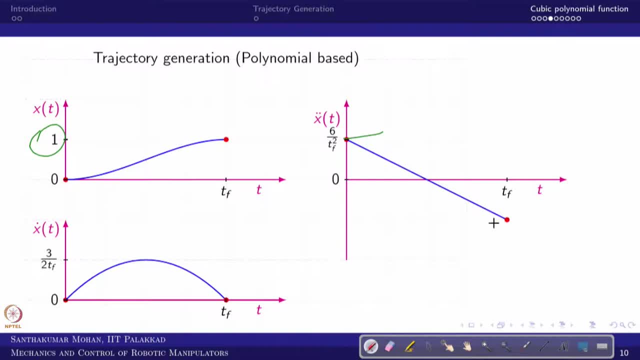 that the acceleration is actually like non-zero at initial phase and non-zero at the final and zero acceleration at middle point. So here actually, like you can see, the middle point, it is actually like. this curve is actually like making another parabolic, So it is actually 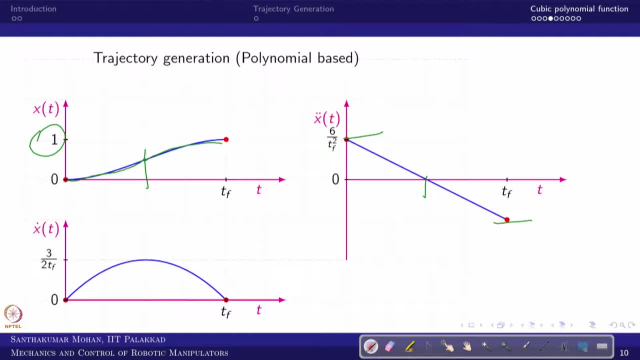 like positive parabolic and this is negative parabolic kind of thing It is generated. So now this is actually like, if you proper, what you call cubic polynomial. this is giving a smooth profile and it is actually, like you can say, twice differentiable. in that sense this is one of the easiest way to apply. So most of the industrial manipulator. 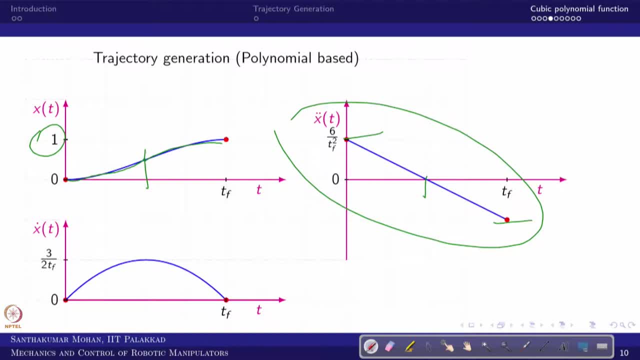 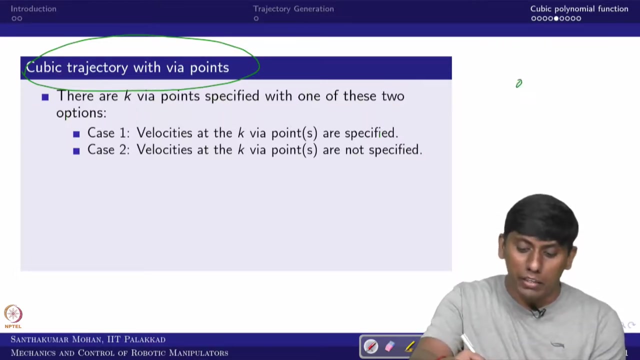 used cubic polynomial. that is why we straight away started talking about this. But the problem here is we do not have any control over the initial and final acceleration. So if you want to want to, One is this what you call via point velocity also specified, then that would give actually. 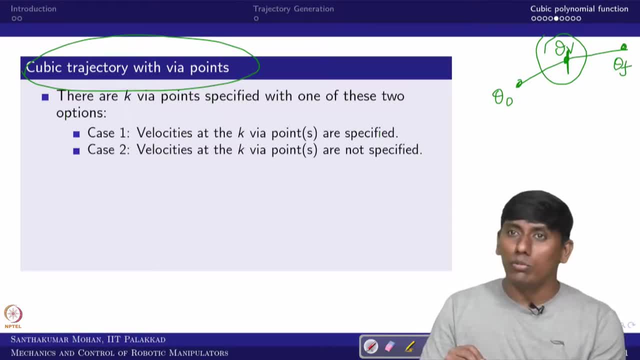 like you can say 8 equations and 8 unknowns and you can actually like solve it and that would give slightly a trickier way that we will be seeing in the next slide. But the other one is actually like the velocity of the you call the via point is not specified. 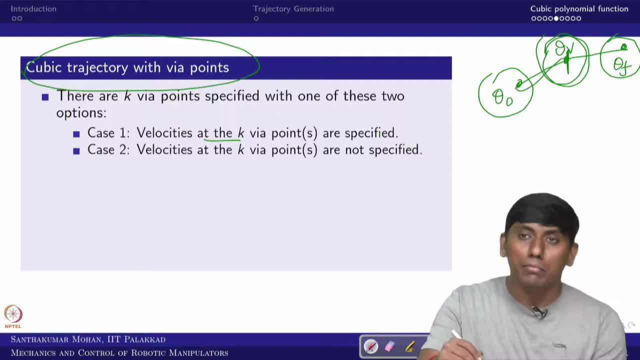 then we can see that the velocity is what generated from here, that we can continue as that is the velocity. So in that sense the initial acceleration and velocity of the second segment would be the final acceleration and velocity of the first segment. that way we can equate So that 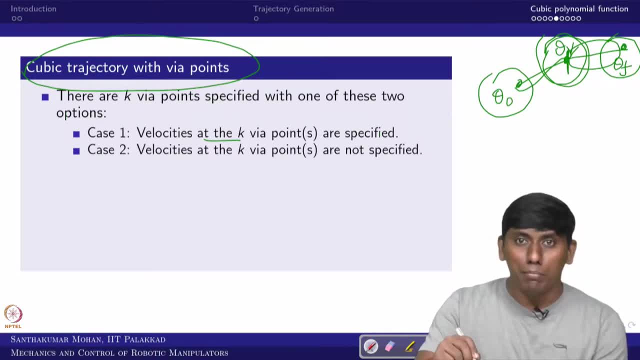 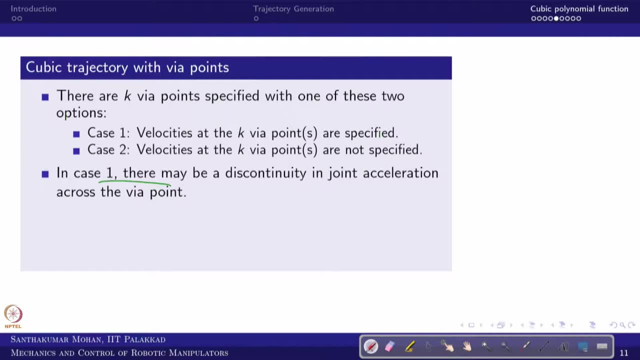 would give further add on that make life simple, okay, So that is what we are trying to see. So in that sense you can see the. in the case one, there may be a discontinuity because you are specifying the, what you call the via point velocity that make the joint acceleration. 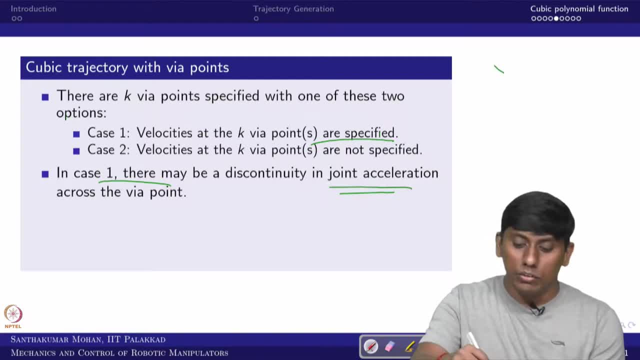 So in that sense the initial acceleration is actually like jerky. So in the sense, so it end here and another one end somewhere, like this: So this is the first segment and this is the second segment may come like this: we can see that. So this is actually like: 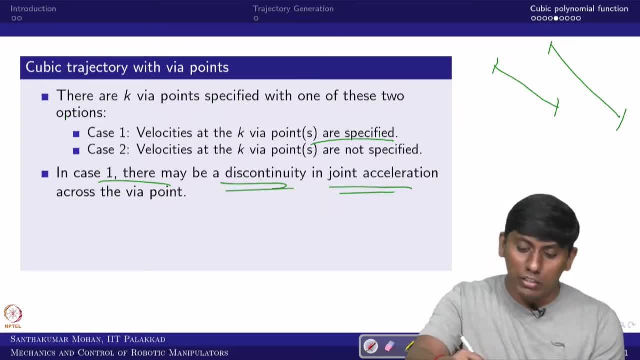 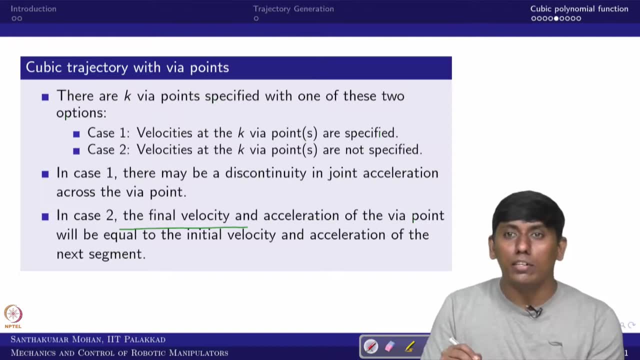 going to give a discontinuity, which is not encourageable. So, in the sense, this point is discontinuous happening, okay. So, whereas the second one, the final velocity and final acceleration of the via point, would be equal to the initial velocity and acceleration of the second segment. 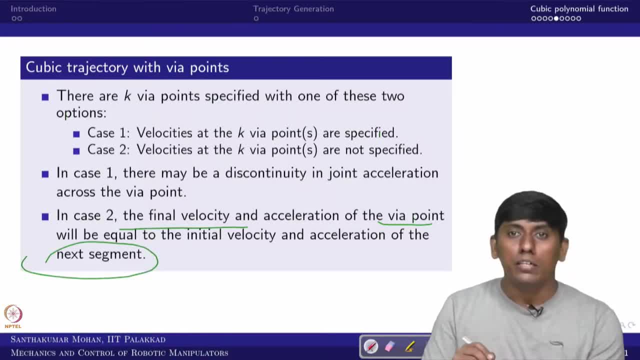 So in the sense, we can actually like use this way. So in that sense it is actually like give the smooth transition and as well as the acceleration would be, for example, this way. So it comes like this, it goes okay, there would not be any discontinuous happen. we can. 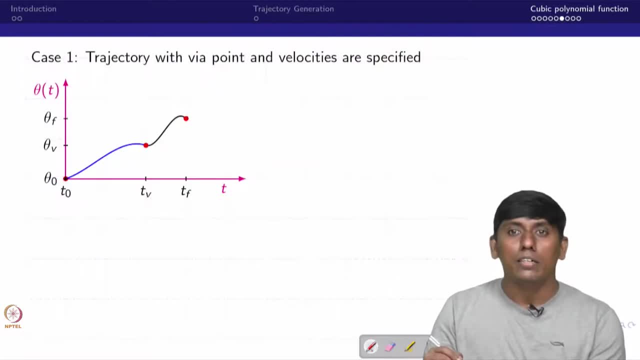 see that how it actually like happening it right. So in that sense we take the via point segment, So you can see like we take first one with velocity specified. So then you can see like this is actually like solve as like independent cubic polynomial. then this is: 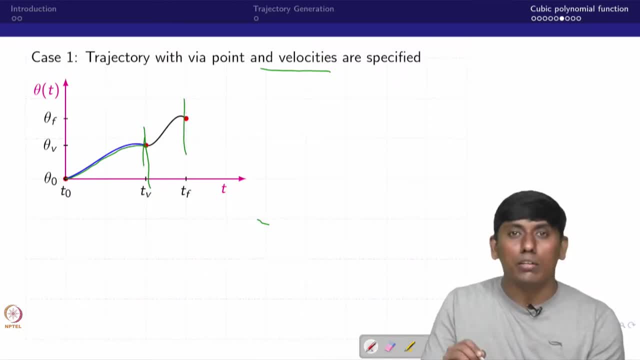 actually like solve another independent cubic polynomial and you can actually like use it So in the sense. so you have first set of equations, so t0 to tv, okay. the second segment is actually like tv to, so tf. So that way will make it so in the sense. x of you can say t would be. 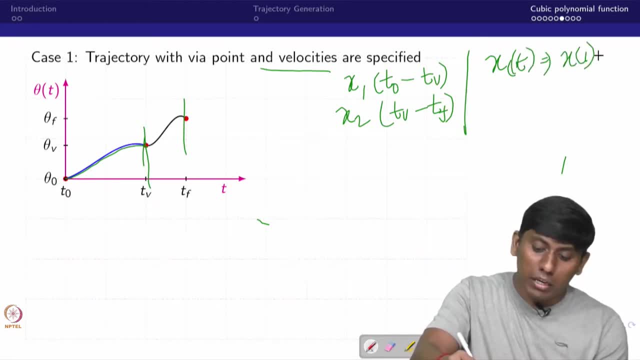 contained actually x of 1. Y, 1. S, 2. S, 4. actually like the first duration, So T 0 to T v and x of you can say 2, that would be. so T v to T f. ok, So like that we can actually like use it. So in that sense you have actually 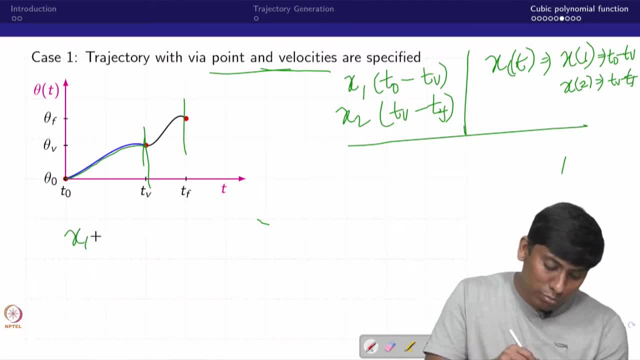 like via point velocity. So in the sense I said that x 1 of T 0 is actually like x of 0 and x 1 dot of T 0 is so x dot of 0, ok. So x 1 of T v is x v, ok. So in this case, 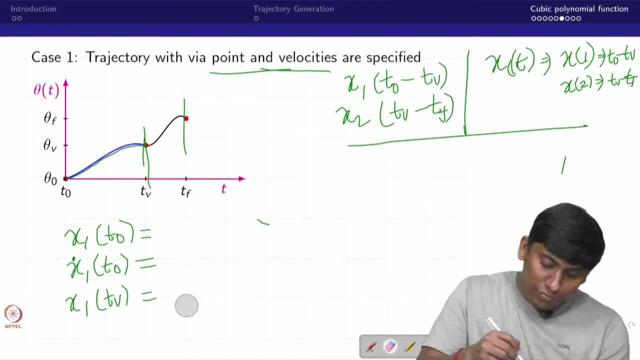 it is actually like I will write it consistent. ok, So I will just use the consistent in the sense I will write So theta. I will write this again: So theta. you can say T 0 and x is actually like theta 0 and theta dot. T 0 is actually like theta, dot, 0 and theta. 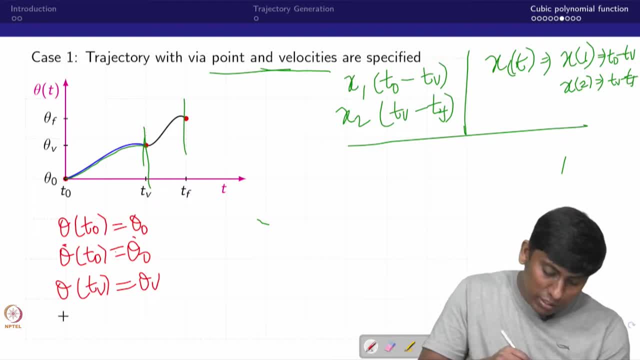 of T v is theta v. ok, So theta of T v is defined like this: ok, So second segment is actually like: so you have 6 variables, So second segment is actually like T f, which is you call theta f, and 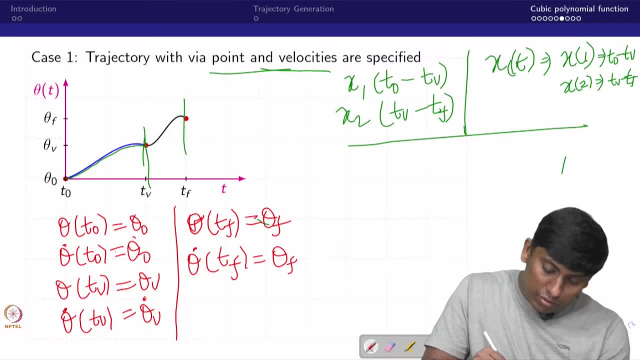 So these all 6 variables would be given, but based on this, how many equations you can generate? So you can actually like: take this is the first segment, So then you can actually like make it. So then the second segment can actually like: do it. So in that sense you will get. 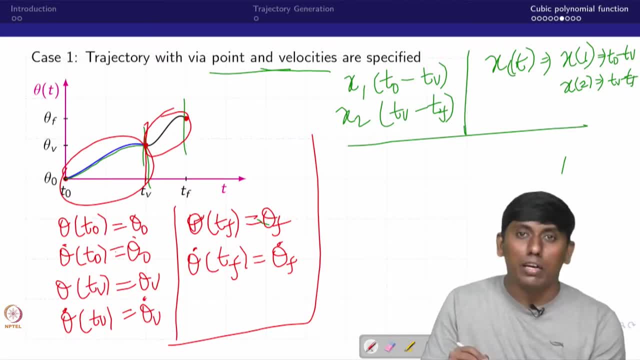 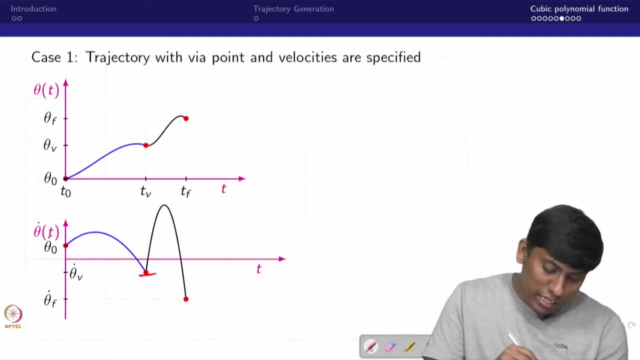 8 unknowns and 8 equations. you can solve it. So the profile will come like this. So based on that velocity you can see. I already said there is theta dot v exist, So you can see like it is. first curve is: 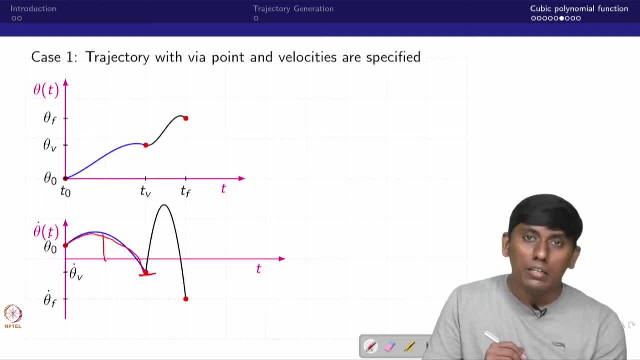 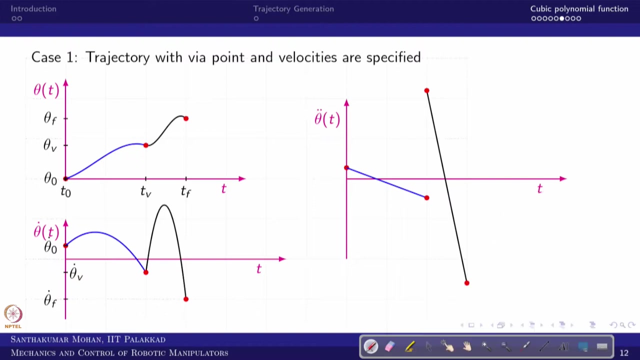 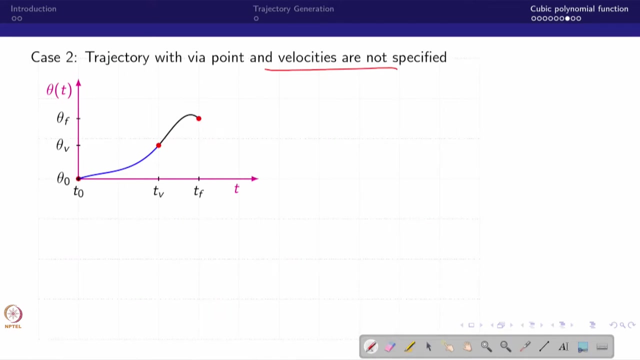 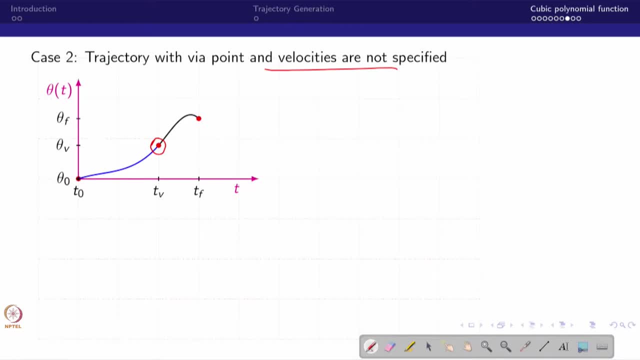 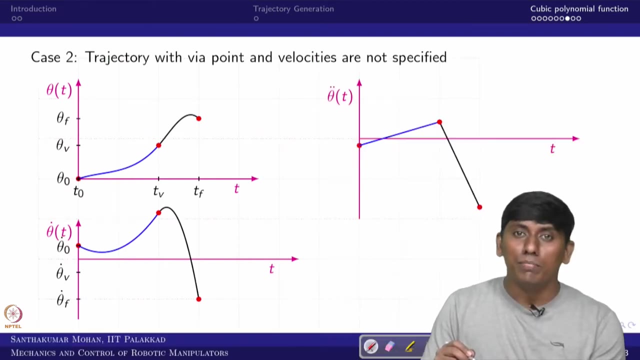 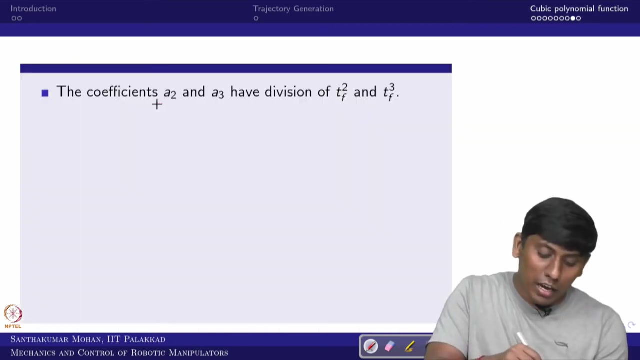 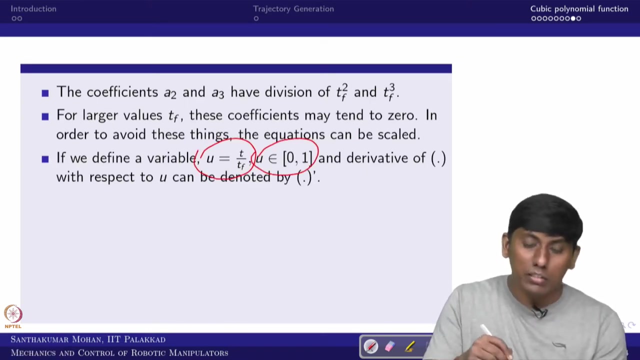 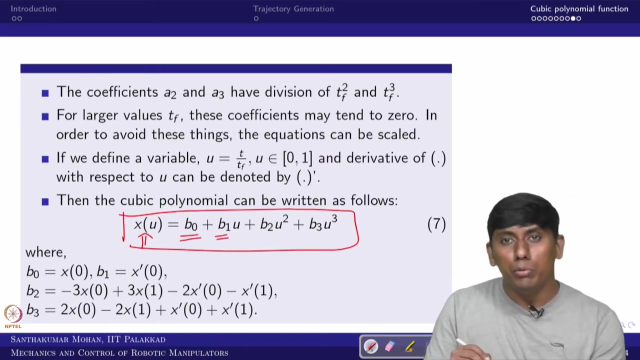 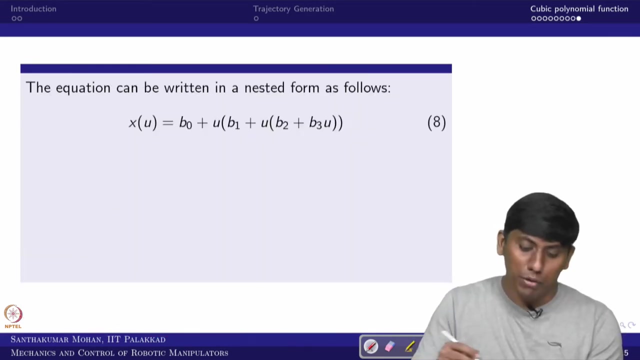 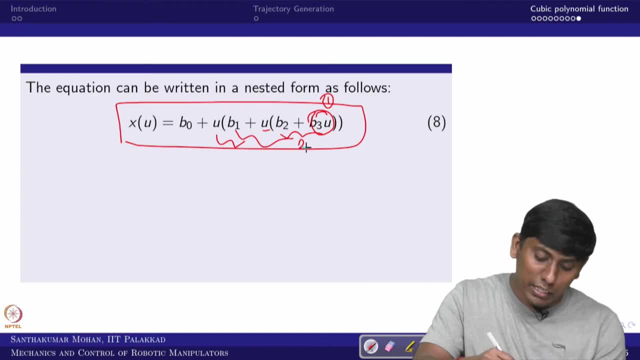 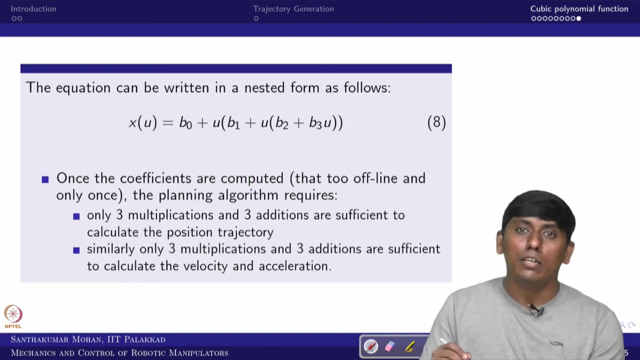